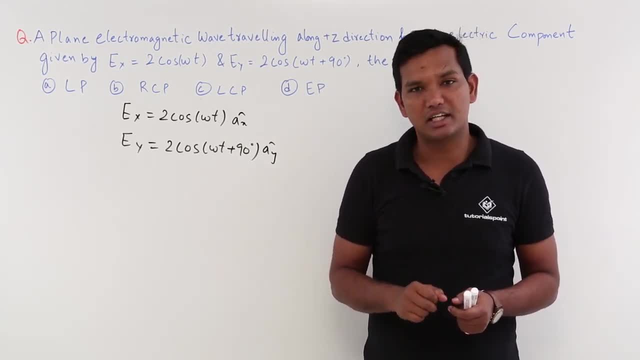 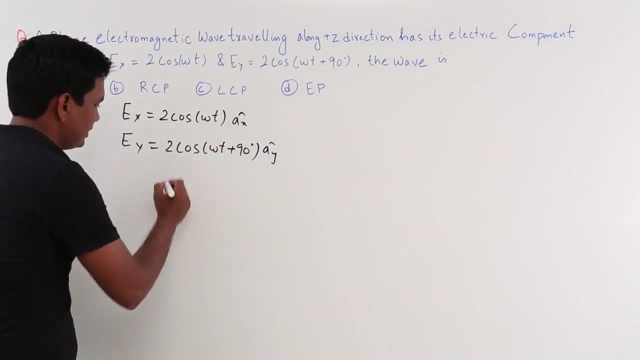 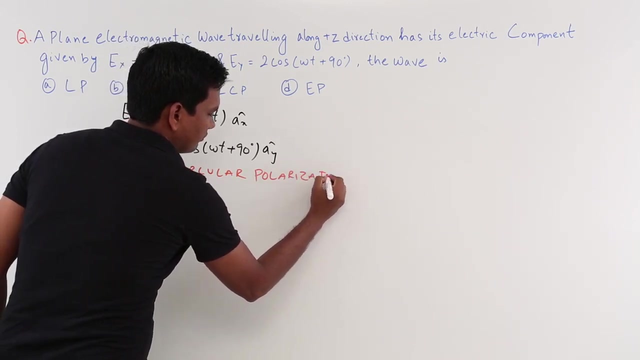 is 90 degree. it is very much clear. it is an circular polarization. So this problem is on circular polarization. So what we have concluded is: it is a circular polarization. This is very much clear. The next part is: as the phase difference between the two components is 90. 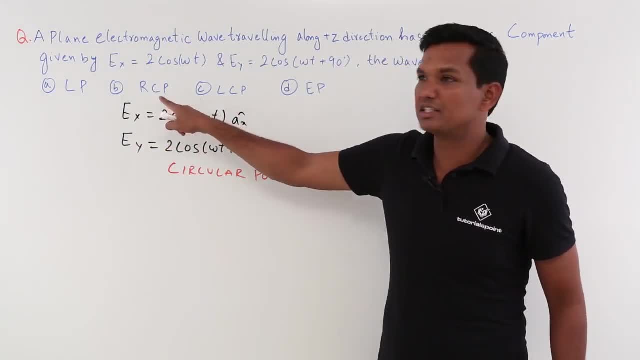 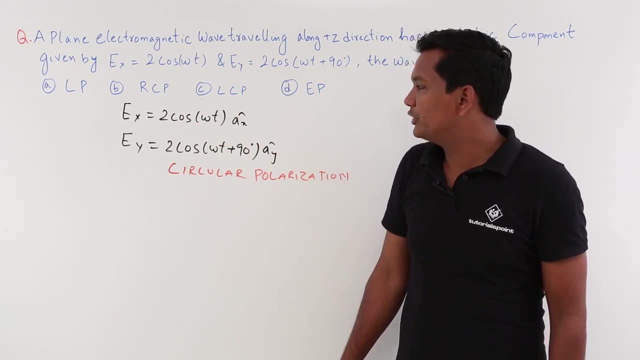 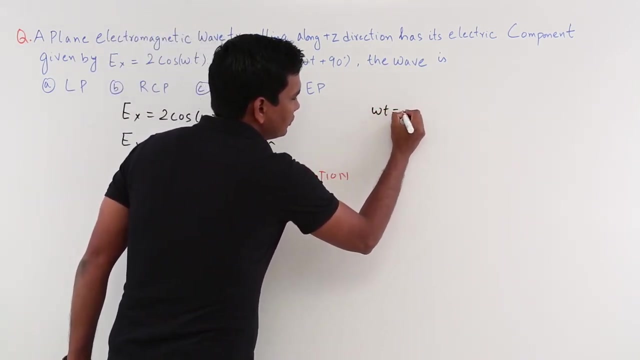 degree. the question says that, whether it is a right circular polarization or left circular polarization, Now we have to identify which type of polarization it is ok, How we can do that. What I am going to do is I am going to plot something. omega t equal to 0, omega. 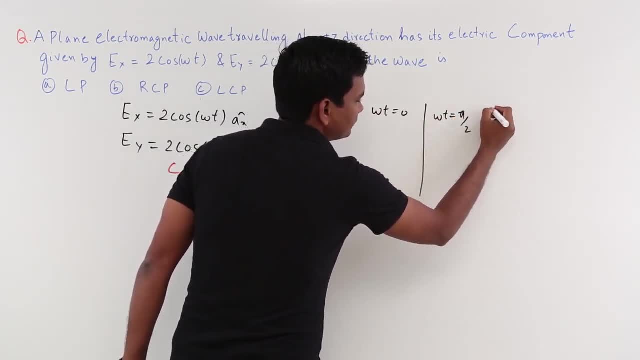 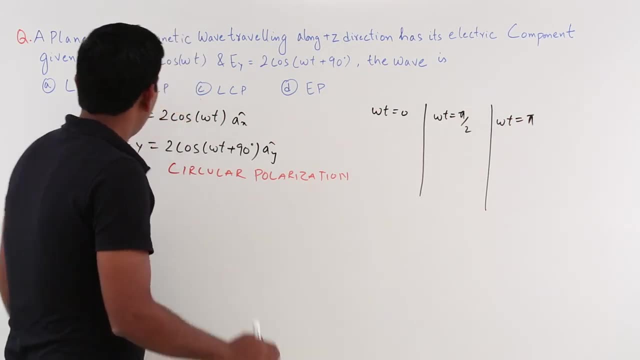 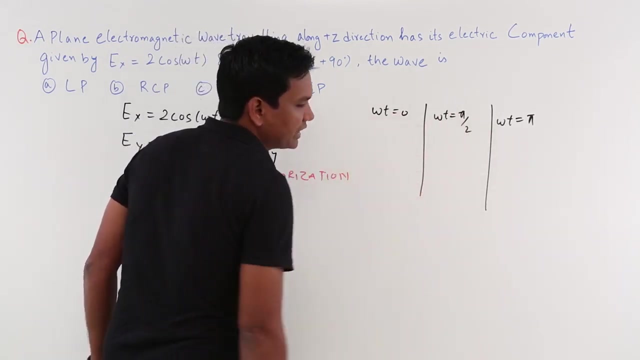 t equal to pi by 2, right, and there is something: omega t equal to pi. What I am going to do is I am going to see the value of Ex and Ey component at omega t equal to 0, omega t equal to pi by 2 and omega t equal to pi- right, When I put omega t equal. 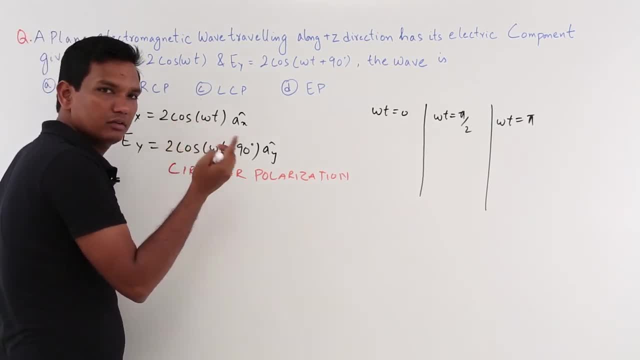 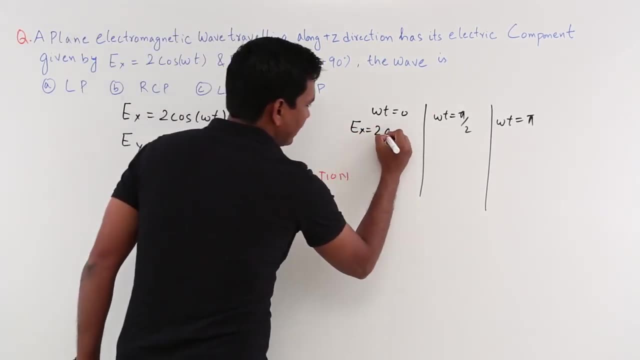 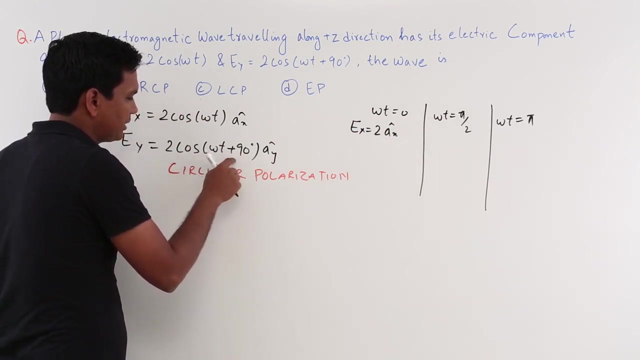 to 0. here what will happen? Cos 0 is nothing, but cos 0 is 1, right. So Ex would be 2, Ex cap At omega t equal to 0, this will become 0, right, and this is 90. So this will become. 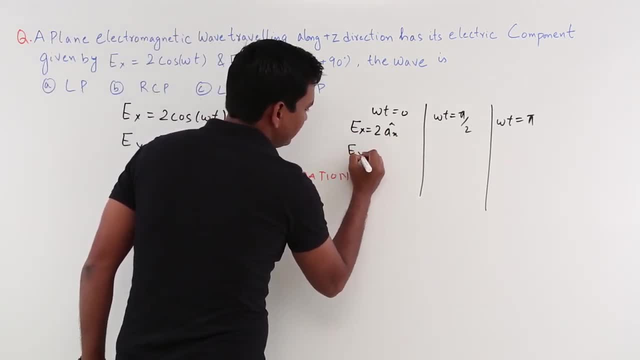 cos 90 and cos 90 is 0. So this Ey would be nothing but 0, right and 0 unit along the, let me say 0 unit along the y axis right, which is same as 0.. Omega t equal to 90.. If I substitute: 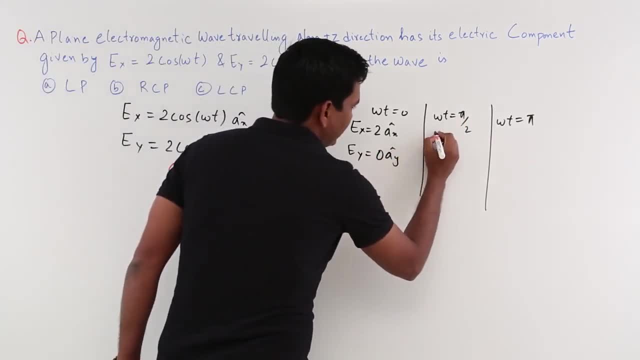 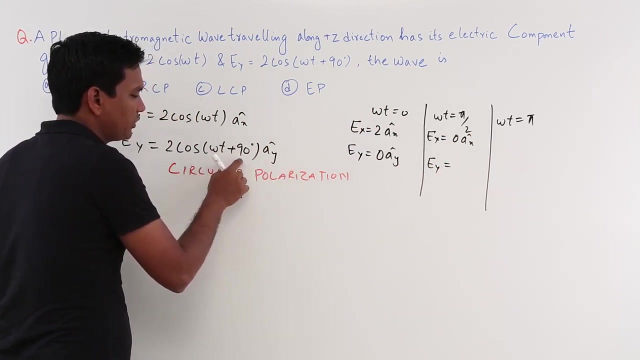 here this becomes cos 90,. cos 90 is again 0.. So my Ex will become 0, Ex cap and Ey will become 90.. Ok, So I am going to substitute omega t 90, 90 plus 90, 180 degree. cos 180 degree is minus 1. So 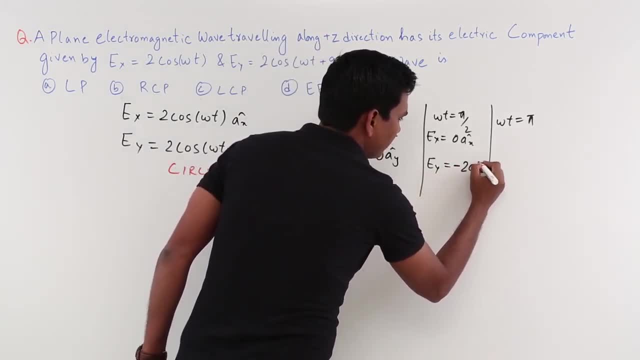 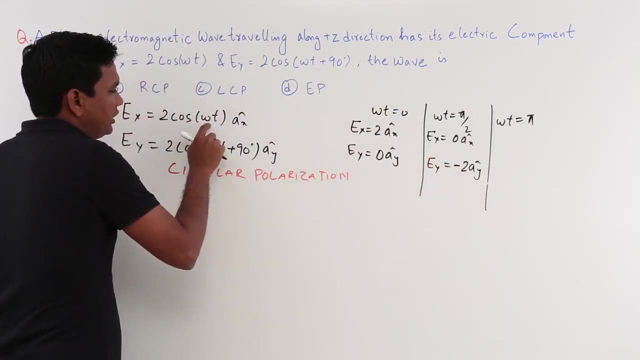 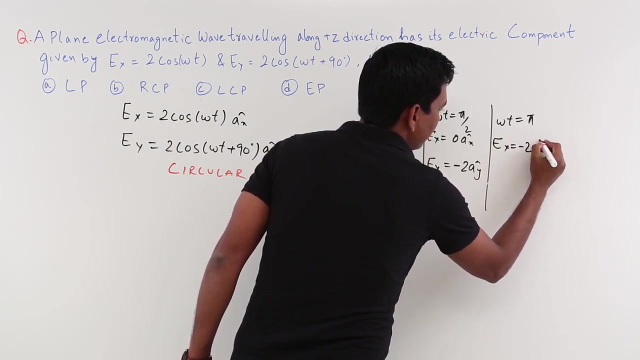 this will become minus 2 ay cap right At omega t, equal to pi, which is nothing but 180 degree right. cos pi is minus 1, right, So this will become ex, will become minus 2 ax cap and ey will. 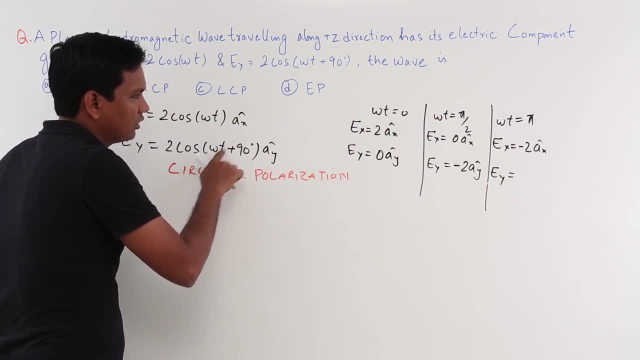 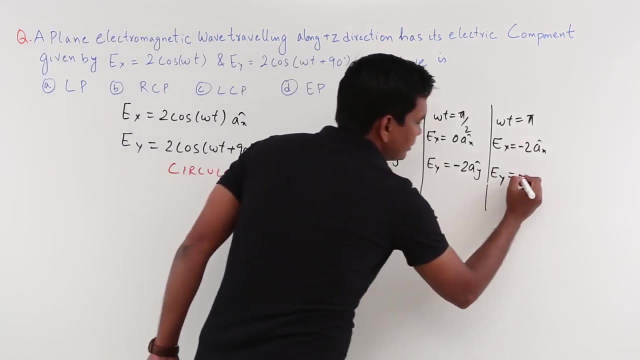 become So it is. pi is nothing but 180 degree. 180 degree plus 90 is 270 degree cos 270, third quadrant 0.. So this would be 0 ay cap right. So I have plot this. just what I have done is: 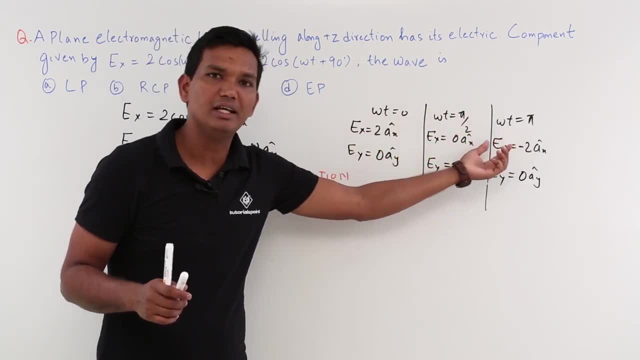 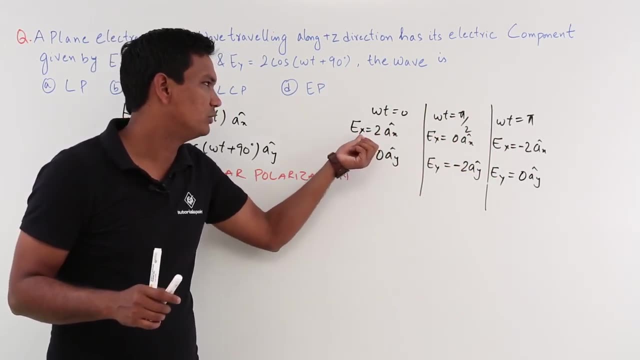 I have put omega t equal to 0, omega t equal to pi by 2 omega t equal to pi And this is the way actually we will be solving. either it is an elliptical or circular polarization And I have put the different components value At this omega t. what will be the component values? 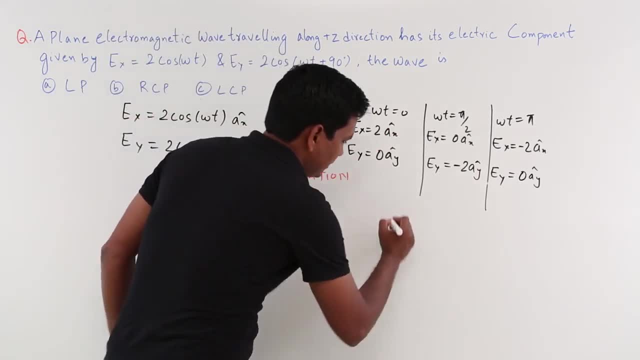 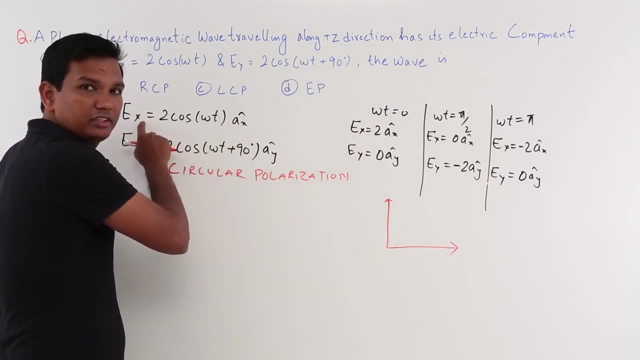 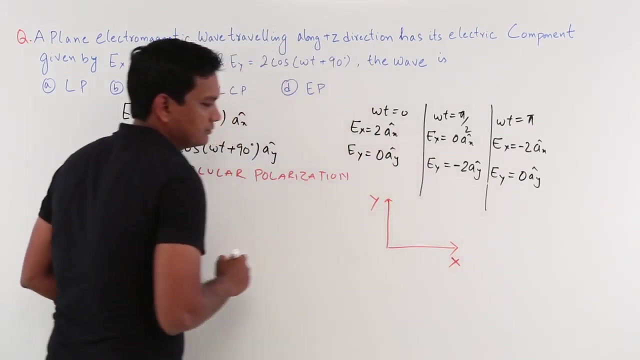 Now let us plot this components. So what I am going to do is: now there is a variation along the x axis. there is a variation along the y axis, right? So let me mark this as an x axis, this as an y axis, right? I am just randomly marked x and y. 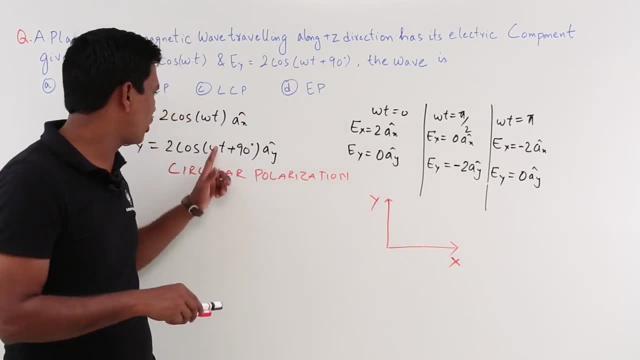 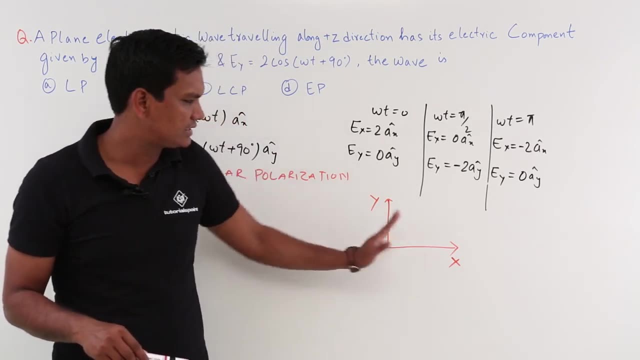 Now, if this is my x, why I marked x and y? Because I have a component along x and I have component along y. If the y sort size there, whatever the component is given to you, you can take that axis. In my case it is x and y. Now, if this is my x, this is my y. where will be my? 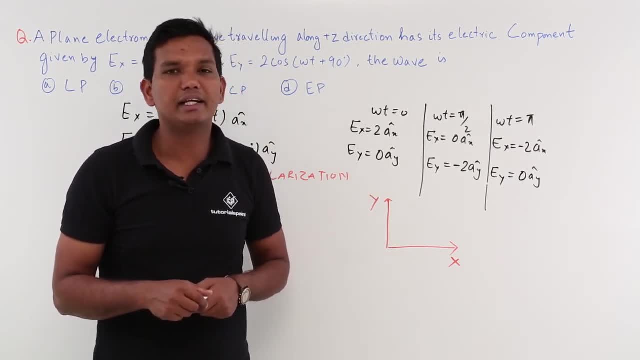 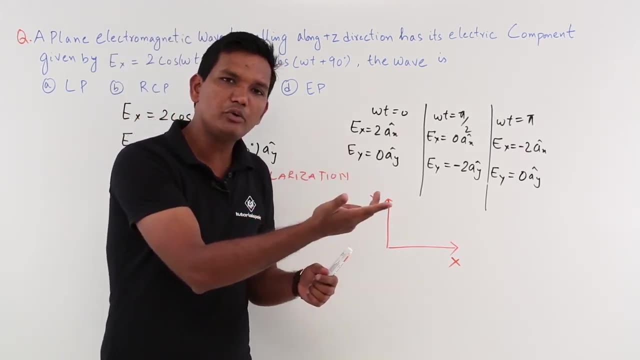 plus z axis pointing right. How I can get that? I can get that by applying the right hand rule. right, We have seen in the previous videos. right, What is right hand rule? You take out your right hand. your forefinger should always point in the direction of x, your middle finger should always 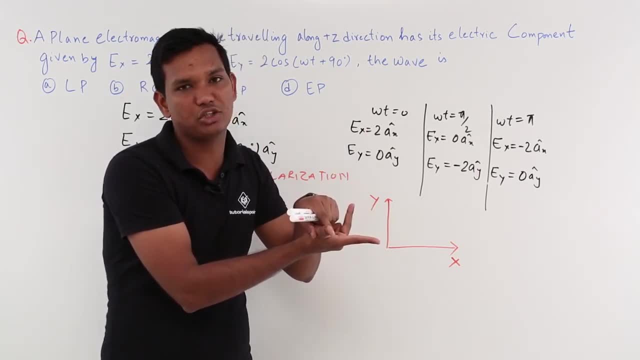 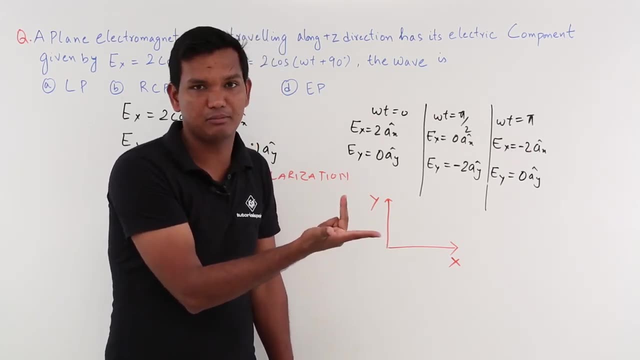 point in the direction of y and thumb should always point in the direction of z. This is what is called as right hand thumb rule. right, So basically, you can take that axis and you can take that axis. So basically, or basically it is also called as right hand coordinate system to be. 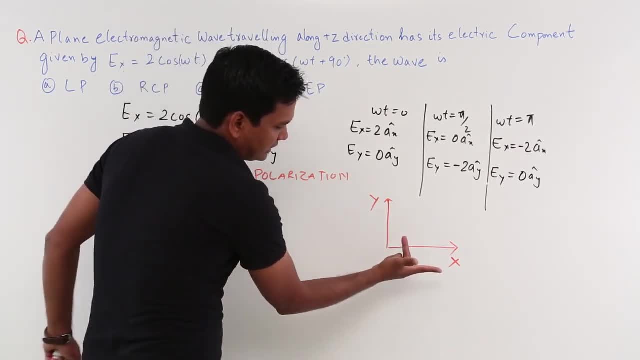 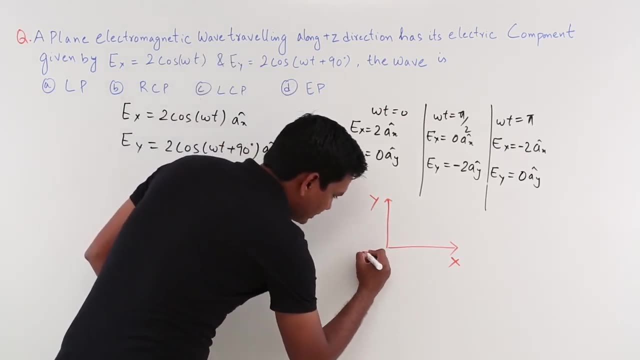 very precise. So if I look like this, you see that this is x, this is y and this is what is my z. It means my plus z is pointing, or I can say that plus z is outside the board. So my z axis. 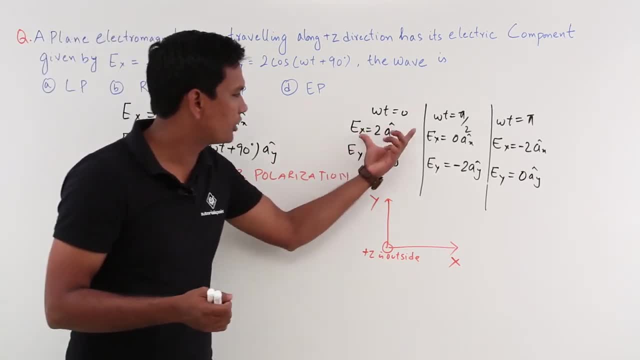 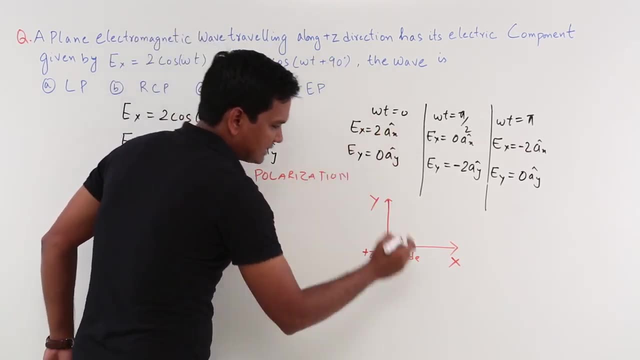 is outside the board. okay, Now I am going to plot these values. okay, At, omega is equal to 0,. I have only 2 magnitude along the x axis, which will be somewhere here right. E, y will be 0. So 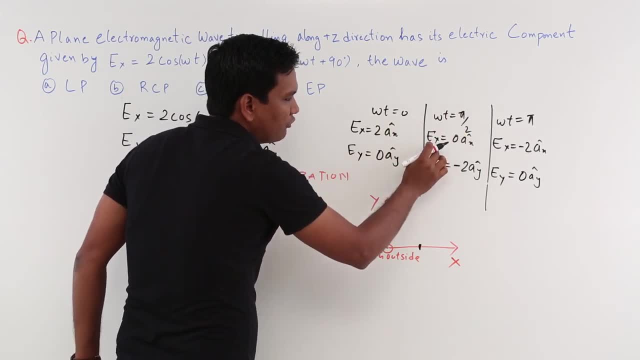 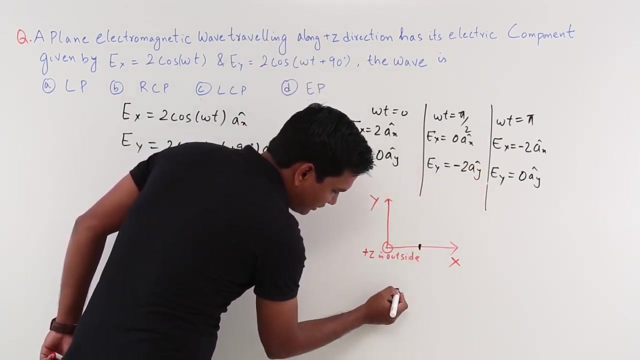 it will be here. no issues Omega t equal to pi by 2,. I have only E y component which will be along the minus y. This is the magnitude remains the same. The magnitude is 2, but it is along the minus y axis. This is plus y axis. It means minus y will be somewhere here, right, If you plot. 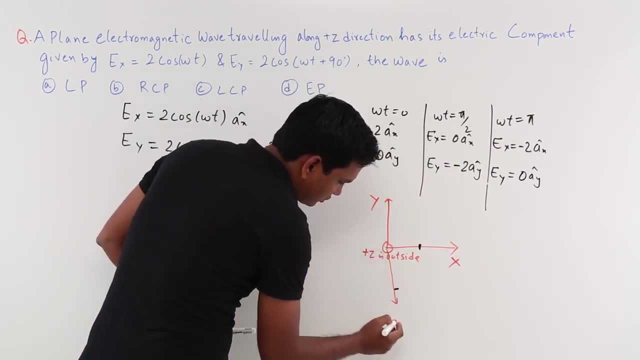 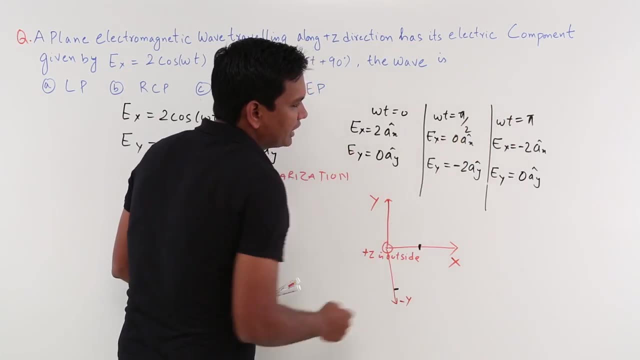 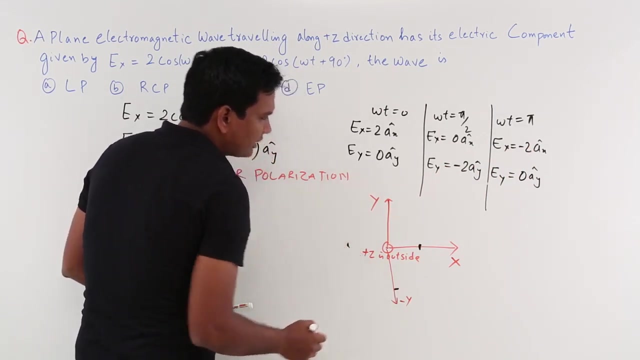 where will be minus y? It would be somewhere here. So this will be your minus y axis, right? Same way, if I go here, at omega t equal to pi, I have a 2 unit along minus x axis, which will be here right again somewhere. So 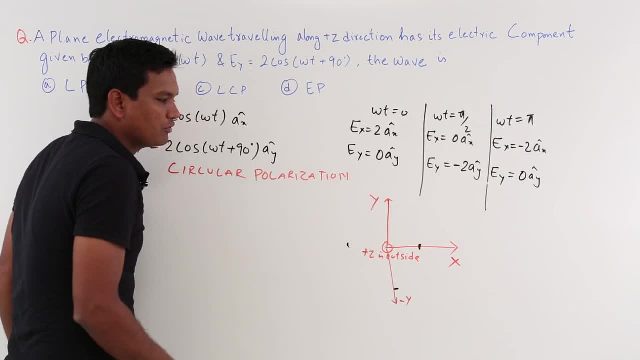 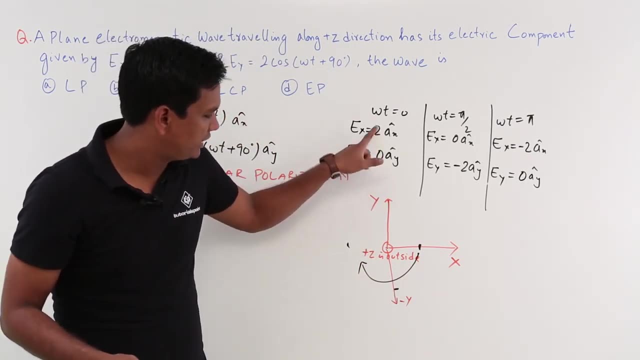 can I say that when I am moving along omega t, what I am observing is I am rotating like this Right. You see that it was 2 a x. So somewhere here I put some 2 magnitude. then you got minus 2 a x. I am rotating like this right. So it is 2 a x. So somewhere here I put some 2 magnitude. 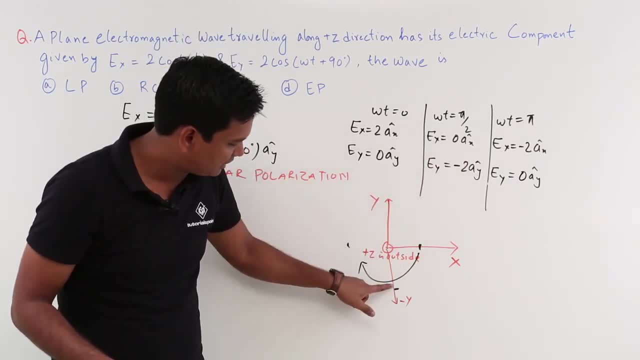 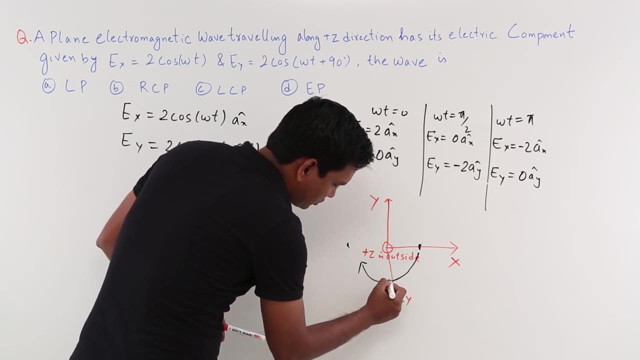 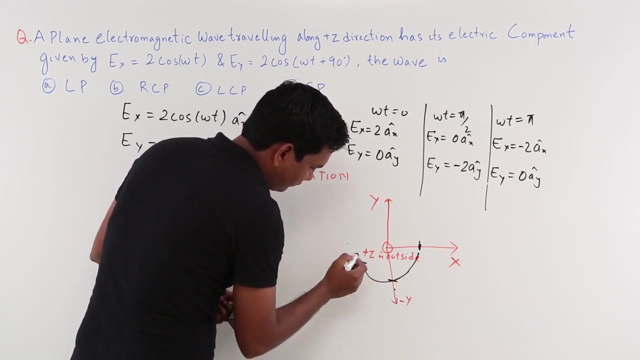 a y, which is nothing but 2 unit along minus y, which is somewhere here. So, basically, to be precise, this figure should be: or this is what is your 2 and this is what is your 2 unit right. and let us say that this is what is your, this is what is your 2 unit right. So this is what it is. 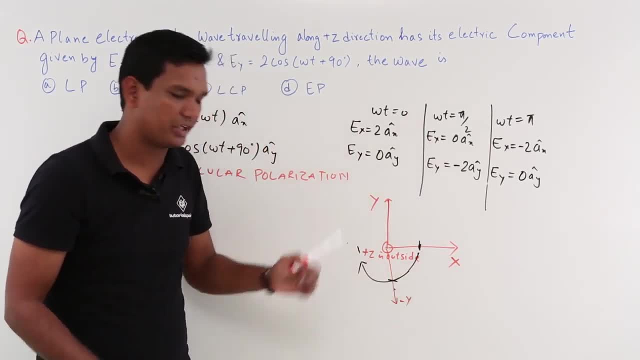 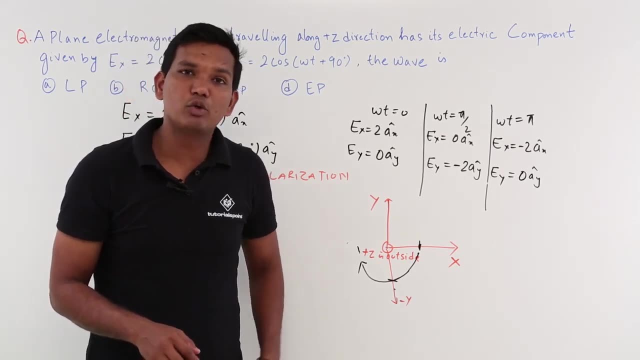 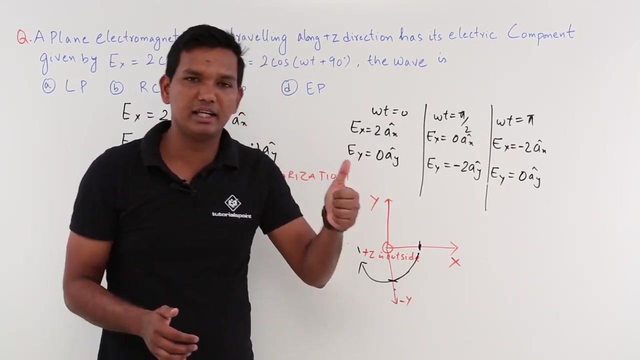 rotating. So, as I am moving, this is how it is rotating. Now, as I have done this rotation part, what I need to do is I have to conclude on whether it is a right circle polarization or left circular polarization. What I am going to do is I have to point the thumb, I have to take the 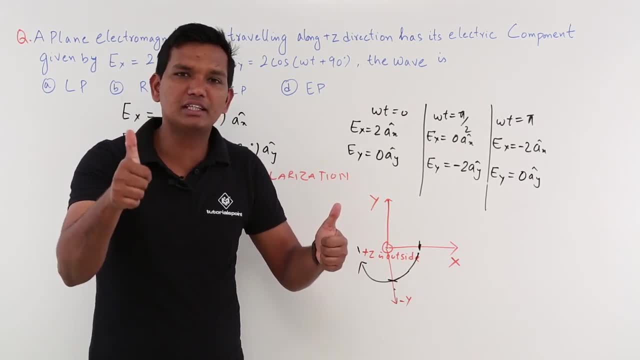 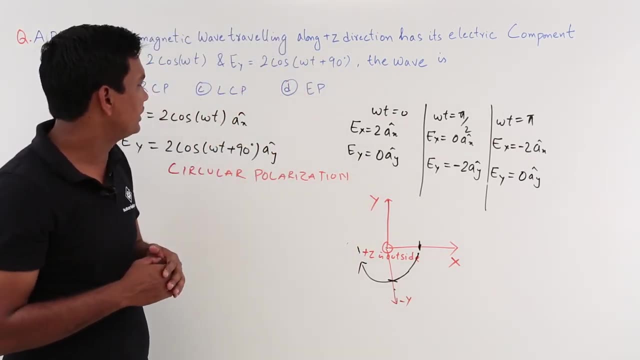 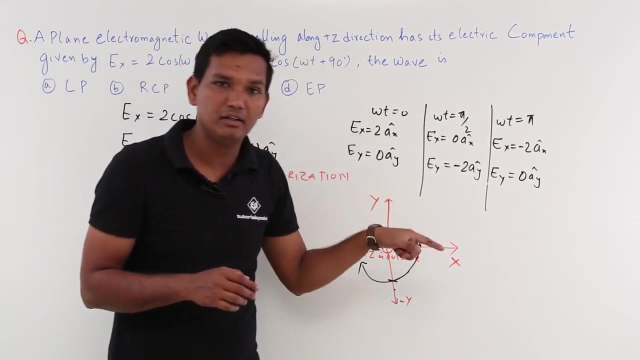 right hand and I have to take the left hand. I have to point the thumb in the direction of propagation. Now, in which direction it is propagating? right Now it is being given in the problem itself- the wave is propagating in the plus z direction right, So it is propagating plus. 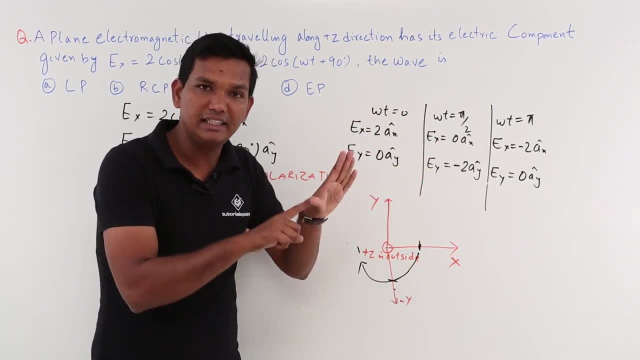 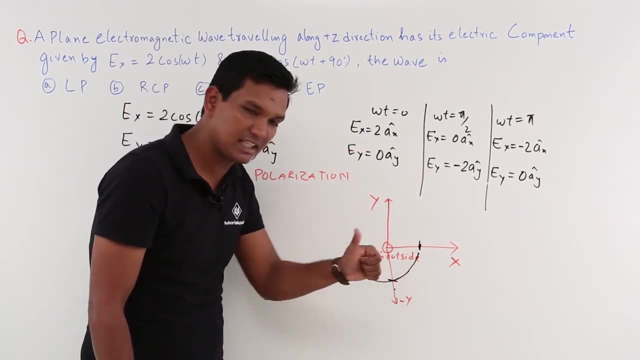 z. So it is propagating in the plus z direction right. So it is propagating in the plus z direction direction. Point the thumb in the direction of propagation. Let me take my left hand and point the thumb. So you know that the plus z is outside right, We know that already. plus z is outside and